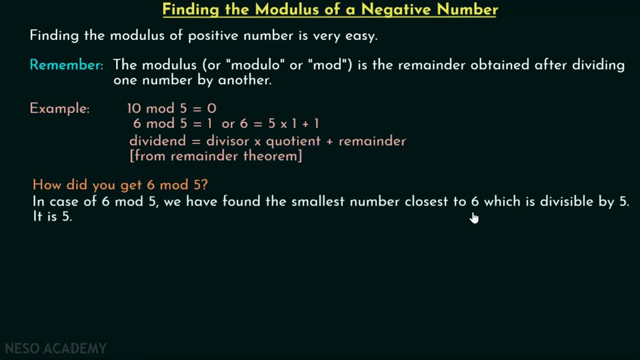 In case of 6 mod 5, we have found the smallest number, closest to 6, which is divisible by 5.. We know that smallest number, which is closest to 6 and is also divisible by 5, is nothing but 5.. Right. 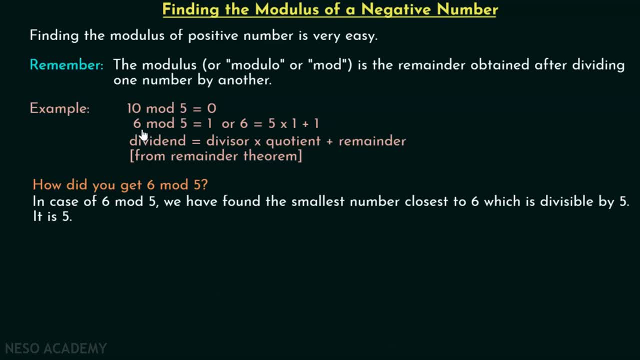 5 is the smallest number closest to 6, which is divisible by 5.. Right, After finding that number, in order to get the remainder, we must subtract 5 from 6.. Right, This 5 must be subtracted from 6.. 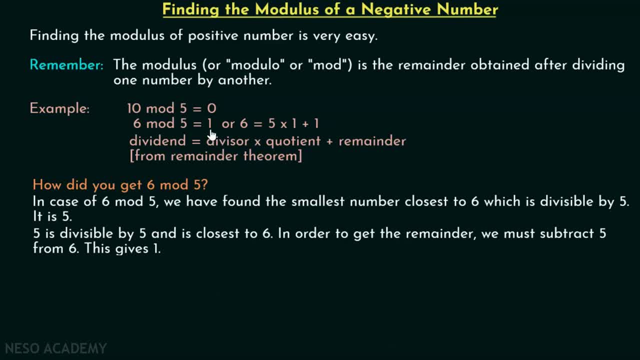 That is 6 minus 5.. 6 minus 5 will give us 1.. Right, That is why we have got this remainder 1. And therefore we can say 6 mod 5 is equal to 1.. Simple to understand, right. 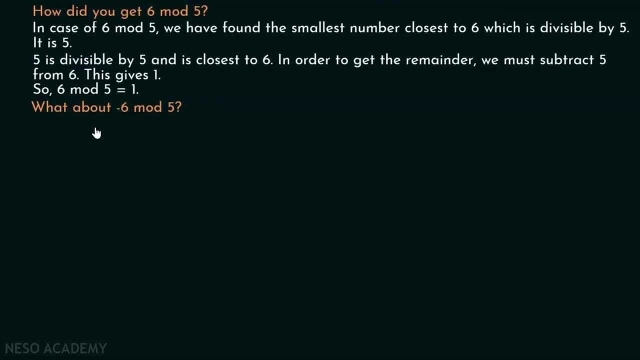 Now, what about minus 6 mod 5?? We have to find the smallest number which is closest to minus 6.. Is it minus 5?? Can we say minus 5 is the smallest number closest to minus 6?? Please note that minus 5 is actually greater than minus 6.. 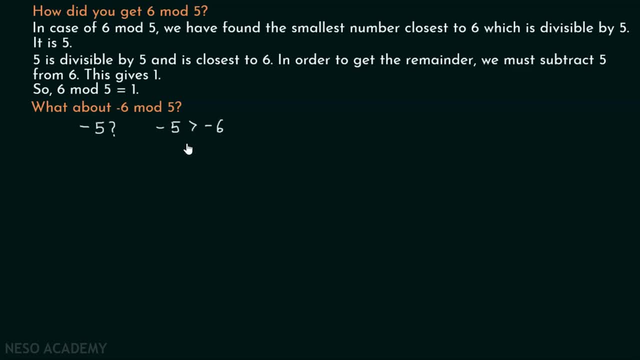 It is not smaller than minus 6.. Therefore, this is not the smallest number closest to minus 6.. Which is divisible by 5.. You can choose minus 10.. The next number must be minus 10, because this number is divisible by 5. 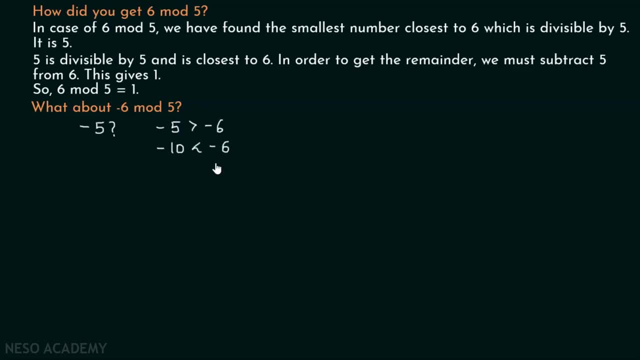 and is the smallest number closest to minus 6.. This is the correct number, Minus 10.. Right After this, the next step is to subtract this number from minus 6.. This means minus 6 minus minus 10.. This gives us minus 6 plus 10.. 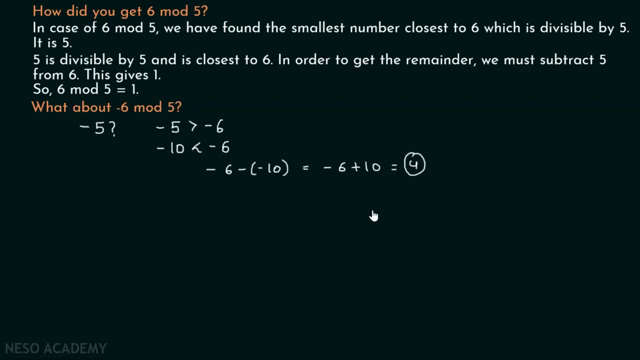 Which is nothing but 4.. Right, So what is minus 6 mod 5?? This is nothing but 4.. 6 mod 5 is 1, while minus 6 mod 5 is equal to 4.. Isn't that simple? 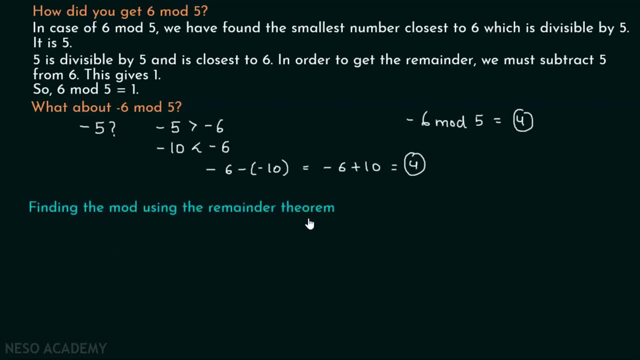 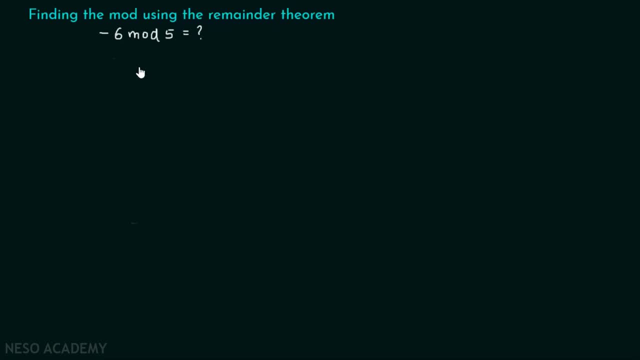 Now let's learn how to find the mod using the remainder theorem. We are interested in finding the mod of minus 6 and 5.. Right, We know that, according to remainder theorem, minus 6 must be equal to 5 into q plus remainder. 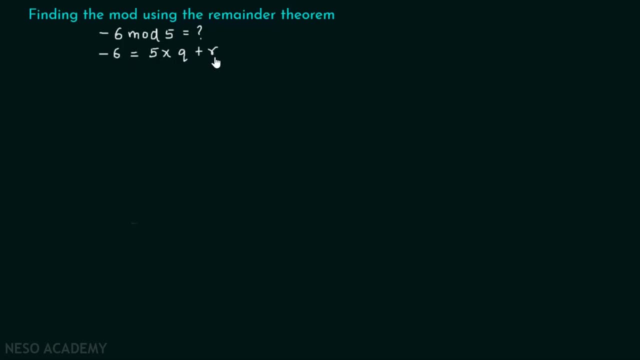 Right Minus 6 is equal to 5. into q plus r. r is remainder, q is quotient. Right Now, we know that range of r, Okay, Range of r- must be between 0 to 4.. Isn't that so? 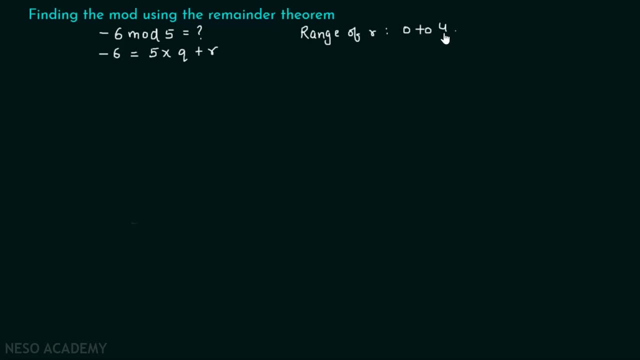 Range of r must be between 0 and 4.. Because our divisor is 5.. Therefore, value of r cannot exceed 4.. Right, We know that r is always positive, But we want the smallest number closest to minus 6,. 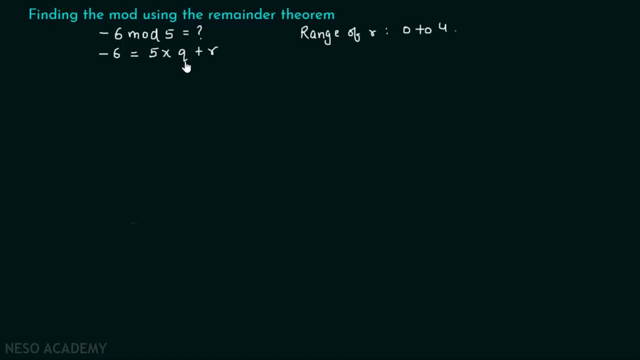 which must be a negative number. Therefore, q must be replaced by some negative number, Right, Let's say q is equal to minus 1.. Let me replace this q value over here- Minus 6 is nothing but 5- into minus 1 plus r. 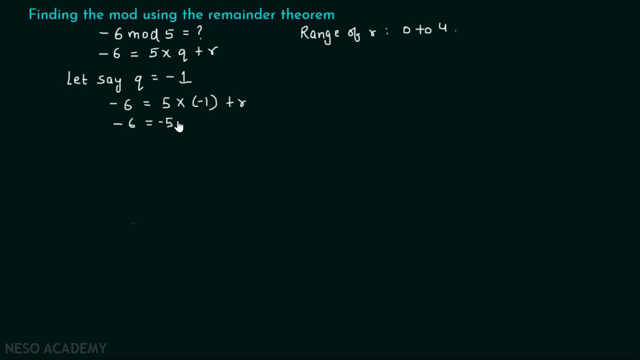 This gives me minus 6 equal to minus 5 plus r. Minus 6 plus 5 is equal to r, Which implies r is equal to minus 1.. Right r is equal to minus 1. r cannot be negative. 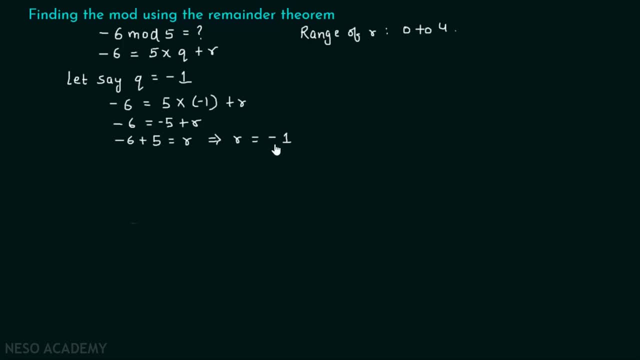 Range of r must be between 0 and 4.. How can r be minus 1?? Therefore, q equal to minus 1 is not correct. Let's say q is minus 2.. In that case, minus 6 must be equal to 5 into minus 2.. 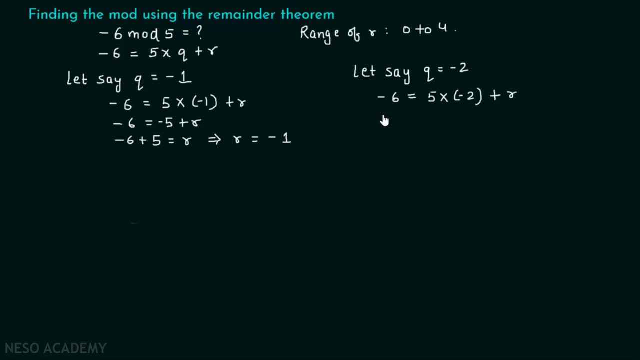 Plus r. Minus 6 must be equal to minus 10. plus r. Minus 6 plus 10 must be equal to r, Which implies r must be equal to 4.. This is the correct answer. Right Because 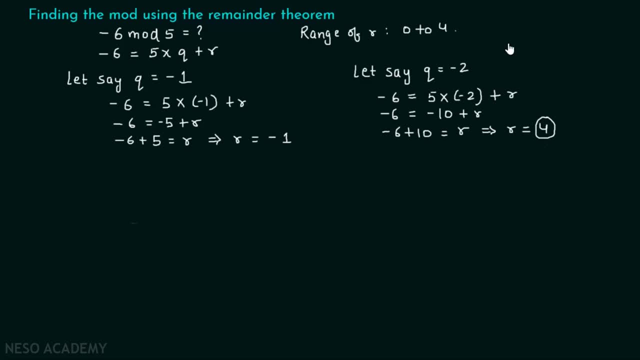 4 is within the range of 0 to 4.. Therefore, it is clear that minus 6 mod 5, 5 is equal to 4.. This is finding mod of negative number using the remainder theorem Right. We have to replace every time this q value. 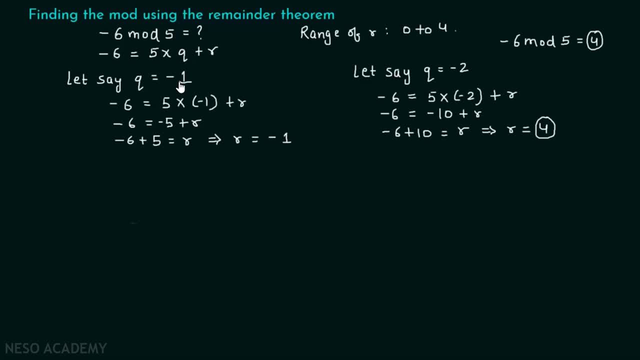 by some negative number. First, we have replaced q by minus 1.. We have seen that remainder is minus 1.. Therefore, this is not the correct value. Then we have replaced q by minus 2.. And after replacing this, 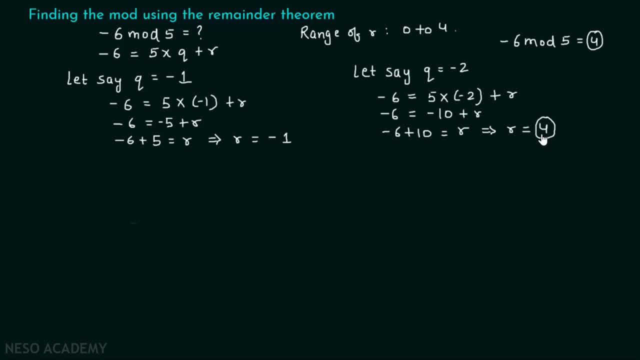 we got this remainder 4, which is obviously the correct remainder Right Now. here is one shortcut method which you must know in order to find the mod of a negative number, Let's say 6 mod 5, equal to r1.. 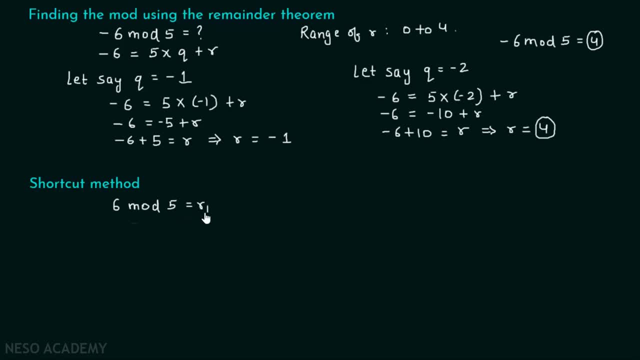 Okay, We know that we can write this 6 mod 5, equal to r1, as 6 equal to 5, into q1 plus r1.. Right, We know that we can replace this q1 by 1.. So this gives us. 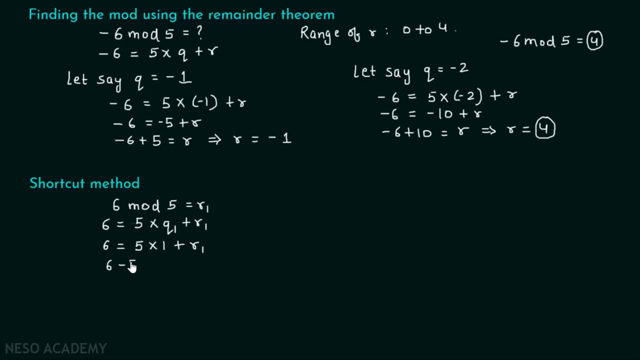 5 into 1 plus r1. And this is nothing but 6 minus 5 equal to r1.. What about minus 6 mod 5? Let's say minus 6 mod 5 is equal to r2.. Here we know that. 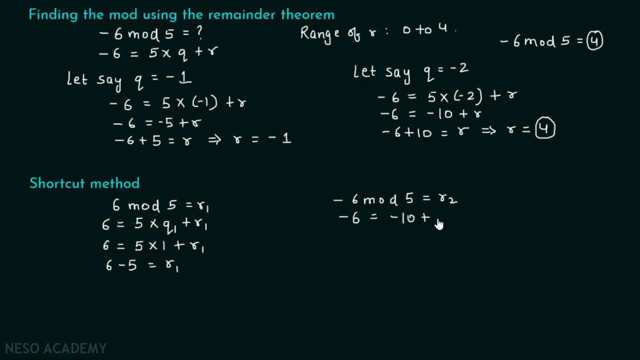 minus 6 equal to minus 10 plus r2.. From here, Right, Minus 6 is equal to minus 10 plus r2.. Minus 6 plus 10 must be equal to r2.. Actually, I want to find. 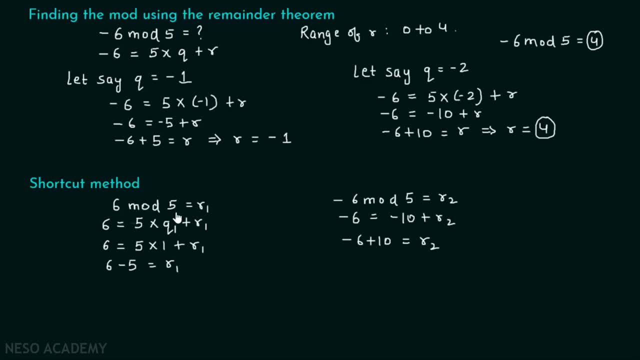 minus 6 mod 5 from 6 mod 5.. Okay, We know that 6 mod 5 is nothing but 6 minus 5.. While minus 6 mod 5 is minus 6 plus 10.. Right Here, this value is similar to this value. 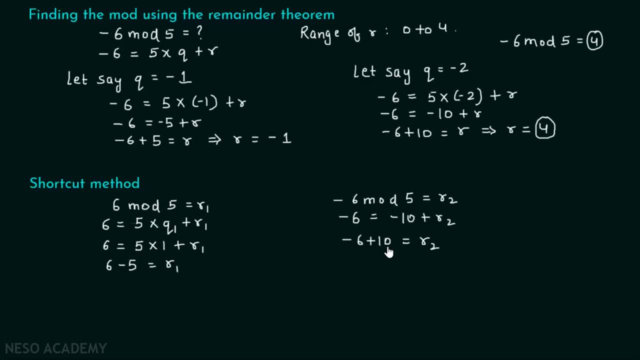 Forget about the signs, But this value is not similar to this value. Here we have 5 and here we have 10.. Obviously, we have to add 5 to this 5, so that we can get value 10.. Right. 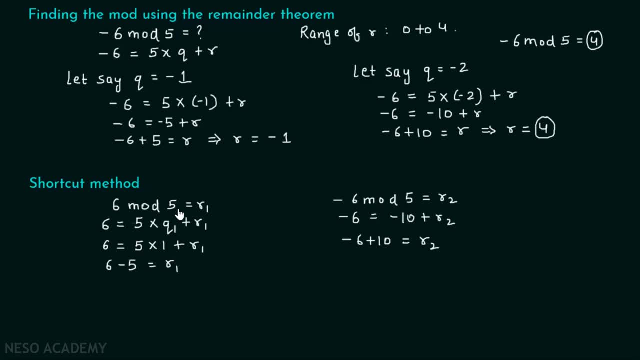 We want to obtain minus 6 mod 5 from 6 mod 5.. Okay, So here, if we add 5 to it, then we will get this value 10.. That means, if we add this 5 divisor to this number, 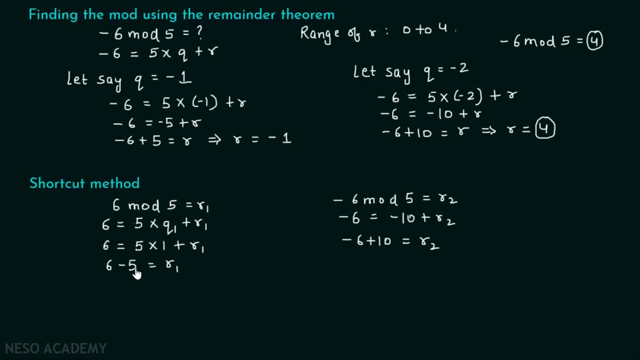 then we will get this number 10.. Obviously this is minus 5.. So here we have to subtract 5 from this. This gives us 6 minus 10.. Obviously, the signs are completely changed. Here we have 6 minus 10.. 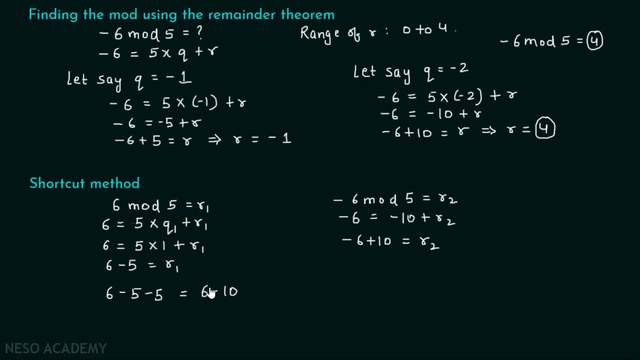 Here we have minus 6 plus 10.. Now we have to change the signs. Instead of doing this procedure, what we can do is we can do something like this: 5 minus 6 minus 5.. Instead of 6 minus 5 minus 5,. 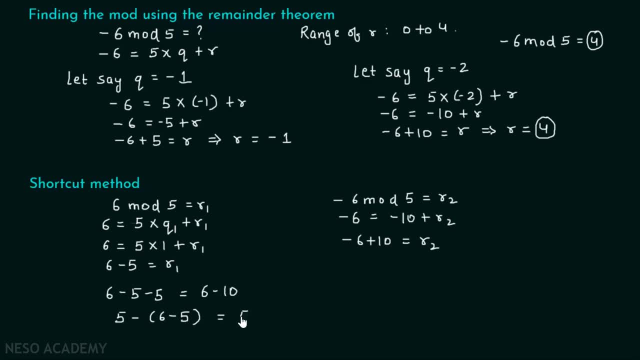 we can do 5 minus 6 minus 5,, which is nothing but 5 minus 6.. Plus 5,, which is equal to 10 minus 6, or in other words, minus 6 plus 10.. Right, This is equal to R1.. 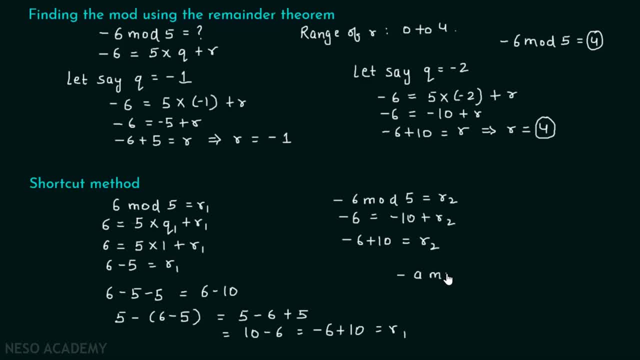 We can generalize this: Minus A mod B is nothing but B minus A mod B, Right? In other words, minus 6 mod 5 is nothing but 5 minus 6 mod 5.. We know that 6 mod 5 is nothing but. 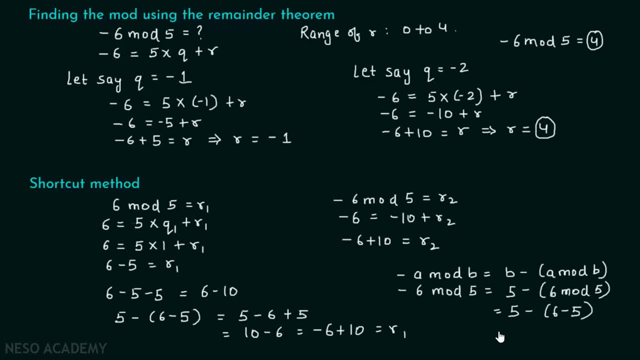 6 minus 5.. And 5 minus 6 minus 5 gives us minus 6 plus 10,, which is equal to 4.. So we can easily find modulus of a negative number from the modulus of a positive number, Right. 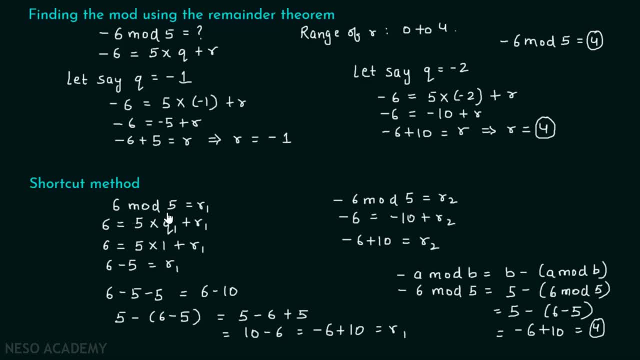 If we want to find minus 6 mod 5, then first we will calculate 6 mod 5. And then we will subtract divisor and 6 mod 5. That is 5 minus 6 mod 5.. That's it. 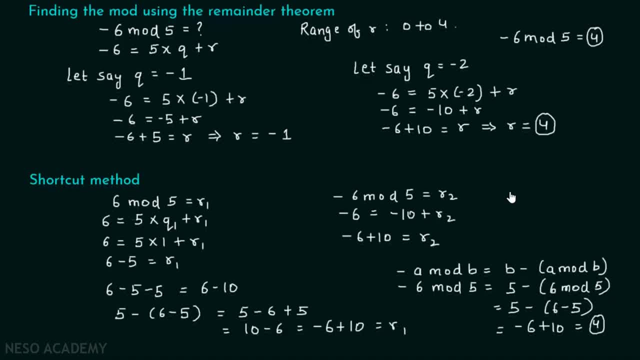 This is the shortcut method, Isn't that? so Now let's see one example. Let's say we are interested in calculating minus 15 mod 7.. Okay, We know that in order to calculate minus 15 mod 7,, 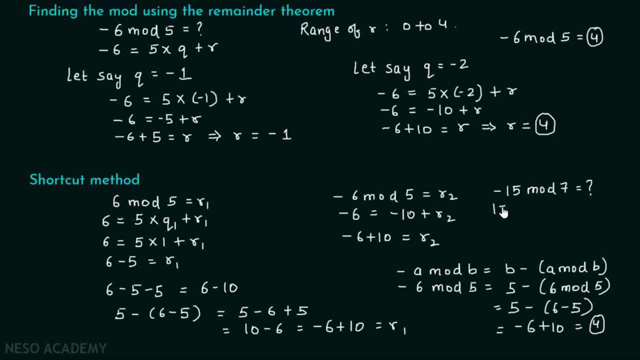 according to the shortcut method, what we can do here. we can find 15 mod 7 first. What is 15 mod 7?? 15 mod 7 is obviously 1.. Now, in order to calculate minus 15 mod 7,, 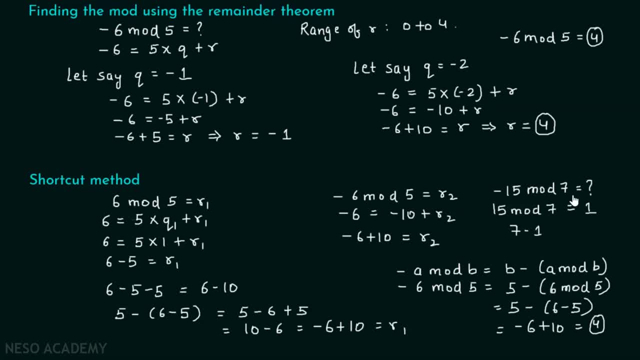 just do this: 7 minus 1.. Subtract divisor and 15 mod 7. That is 7 minus 1, which gives 6.. Minus 15 mod 7 is nothing but 6. Very simple to calculate.